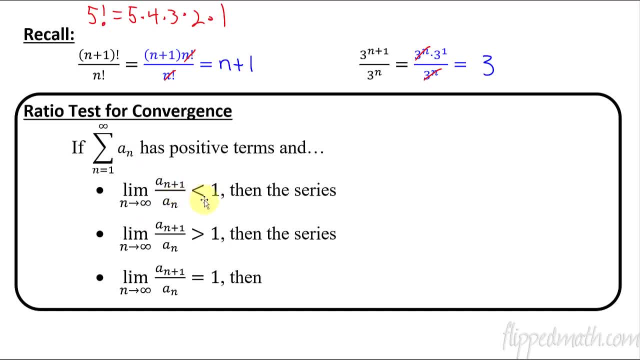 so it's kind of like a horizontal asymptote of this fraction. if that is less than 1, as the limit of n approaches infinity it converges. so if the ratio is smaller than 1, it converges. If that ratio is larger than 1 as you approach infinity, then the series diverges. 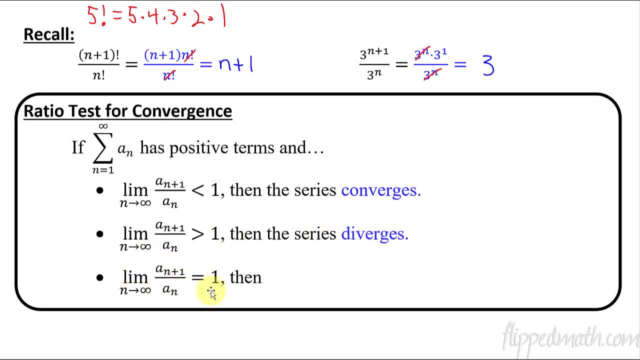 And if that ratio actually equals 1,, well then we've got a little bit of a problem, because if it's less than 1 and it converges, and if it's greater than 1 and then diverges if it equals 1, then we just have to use another test. 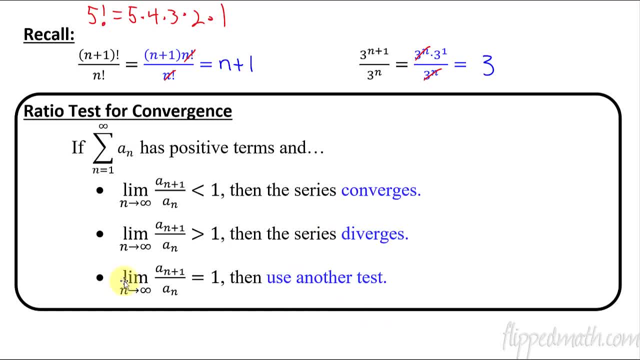 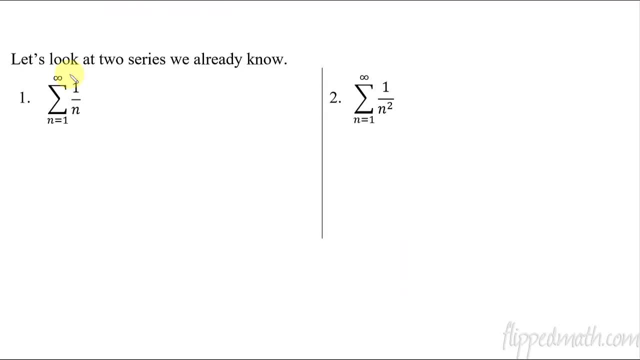 We don't have enough information, so we have to keep working. All right, so there is the main things for the ratio test of convergence. So let's look at a couple. Let's look at a couple of series that we already know, and that is this one here. 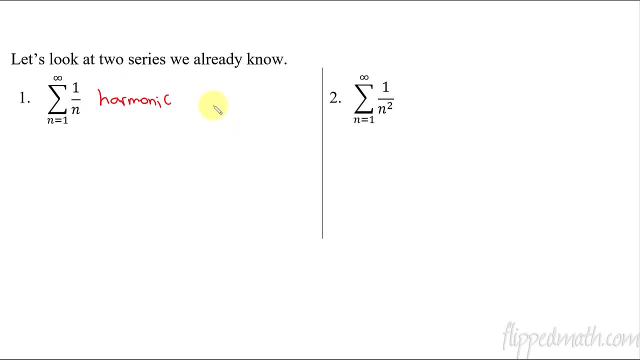 If you remember, this is a harmonic and we've worked with this before when we did p-series and we actually know that this thing diverges And this. we know that one converges. It's a p-series and we know it converges. 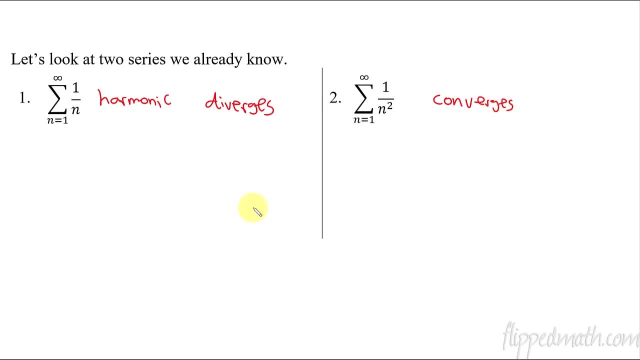 So what about if we use the ratio test with this? Let's see how to work with the ratio test and see what it tells us. So the first thing I do is I'm going to write down that I'm taking the limit of this ratio. 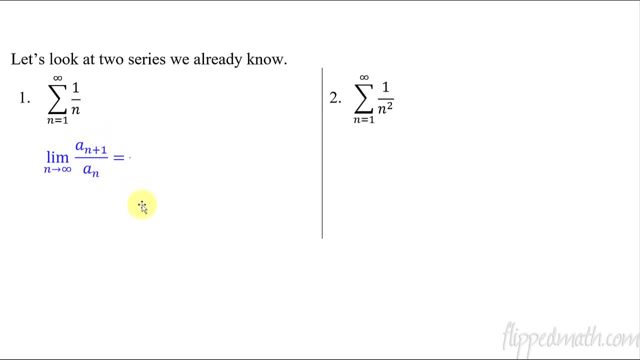 So this is the ratio test, and I need to figure out what that equals. So the next step is: what is a of n plus 1?? That's just plugging in an n plus 1 in there. So instead of an n it's now an n plus 1, and then divided by the original a of n. 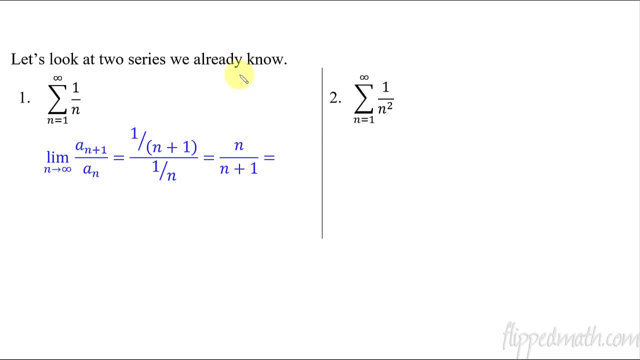 Well, fractions inside fractions, that's like crazy. That's too hard, So I'm going to multiply by the reciprocal instead, which gives me this: Now, my notation actually is wrong. I got a little lazy and forgot to write down that n approaches infinity. 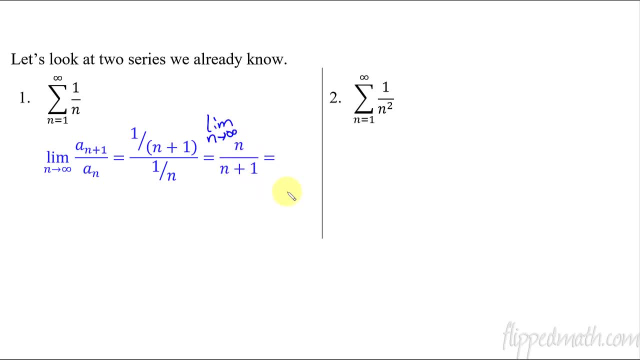 Technically I should have written: n approaches infinity, the limit of this thing. So that's taking horizontal asymptote right. So I have a 1 here, first degree, first degree, So it's just leading coefficients and that equals 1.. 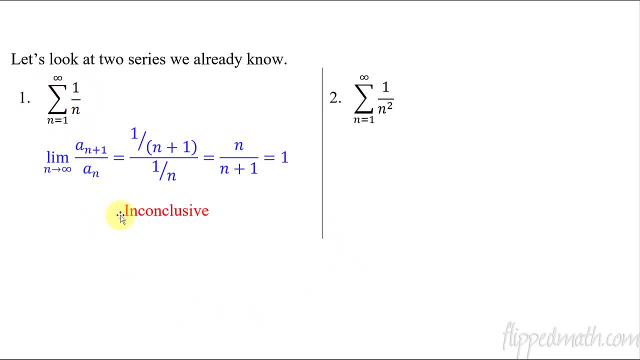 So the ratio test for this harmonic is inconclusive. I can't say anything because it actually equals 1.. I have to do more tests to it. All right, let's try this one. So we're doing the same thing. We take the limit as n approaches infinity of this ratio. 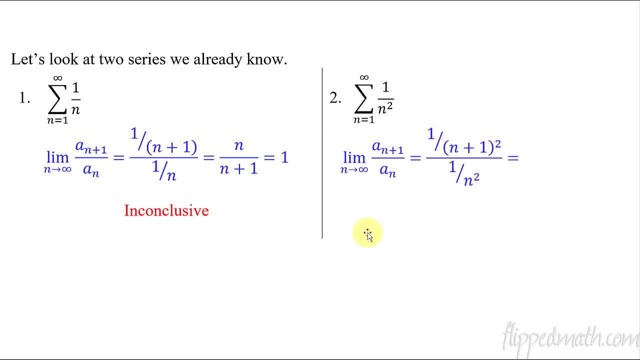 and I plug in an n plus 1 quantity squared On bottom. I still have the n squared. Multiply by the reciprocal instead. Make it a little easier. And then I have an n squared and an n squared. Leading coefficients are 1.. 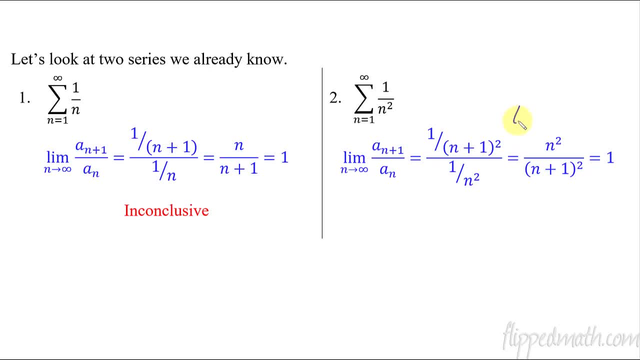 Put them all together. The limit- again, I was being lazy. I should have had in here the limit as n approaches infinity of this whole thing, And then that equals 1.. So what can I say about this? Nothing, I don't know. 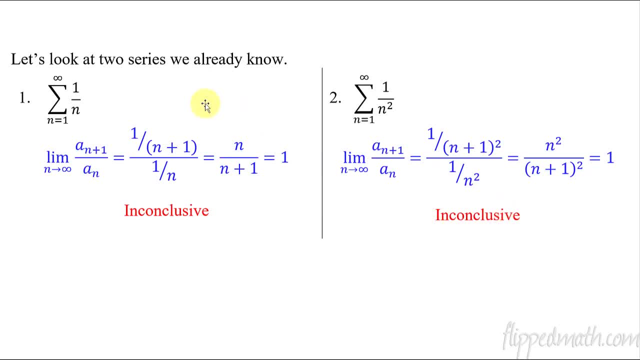 The ratio test doesn't give me enough information for this problem. So what I'm trying to show you is that actually, every time you have a p-series, you can't use the ratio test. It's always going to be inconclusive when you have a p-series. 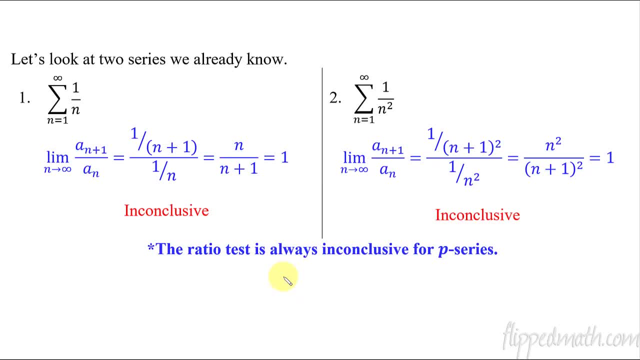 So the ratio test gives you: 1. One more tool in your toolbox of skills to work with series, to figure out if it's converging or diverging. So it doesn't mean you always want to use ratio tests, It just means it might be a useful thing. 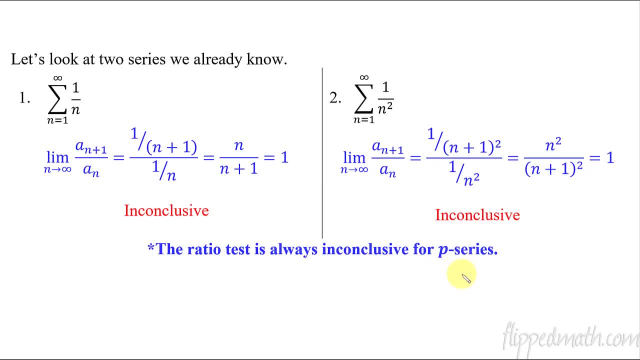 If it's a p-series, you don't want to use a ratio test. You would just use your understanding of p-series and what the degree is on bottom here. That's what the ratio test is going to do for us today. It's just one more thing to work with. 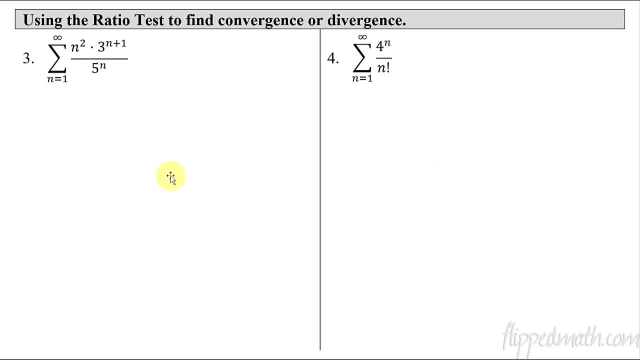 So let's try some examples that do work out that are not equal to 1.. I have found it most helpful that, when you're working through these things, that you first write down what is your a of n plus 1 and what is your a of n. 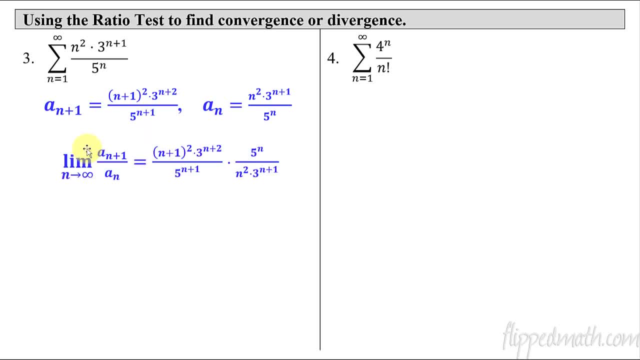 just to make sure you have them both listed. So now, once you have that, now you can start setting up your limit. So limit is n approaches infinity Of this ratio is going to be. so you take the n plus 1 thing. 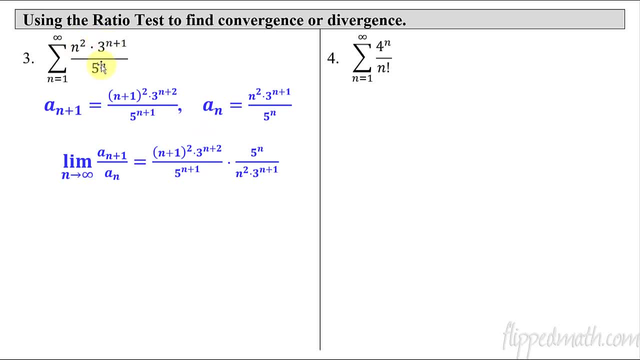 So what did I do? I just plugged in the n plus 1 to the n n plus 1 there. n plus 1 there, That's all this came from. And then you multiply by the reciprocal of a of n. So instead of dividing by that thing, you're going to multiply reciprocal. 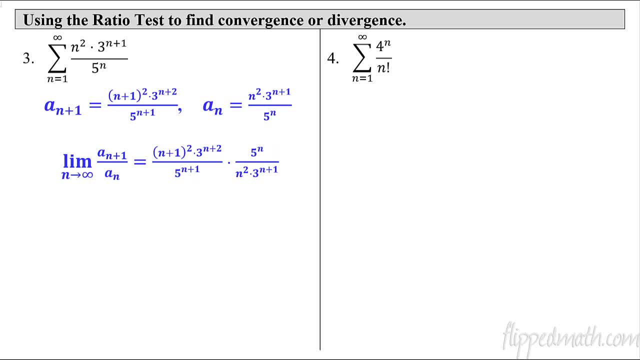 So we'll just do that each time, And then From here you're going to use your skills with exponents to recognize that this 3 to the n plus 2 is the same thing as 3 to the n times 3 to the second. 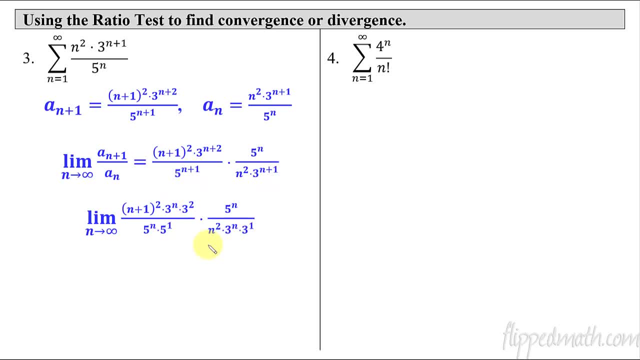 Same thing with this: 5 to the n plus 1, 3 to the n plus 1.. You can see how I broke it all up down there, And now let's try to cancel stuff out. So I've got a 3 to the n a, 3 to the n a, 5 to the n, 5 to the n. 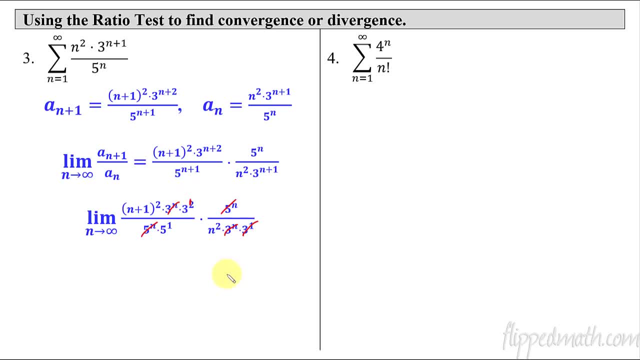 What else 3 to the 1 can cancel with one of those 3s. So then that really cleans up quite a bit. You can see all that stuff is going to cancel, And all I'm left with is this here: n plus 1, quantity squared times a, 3.. 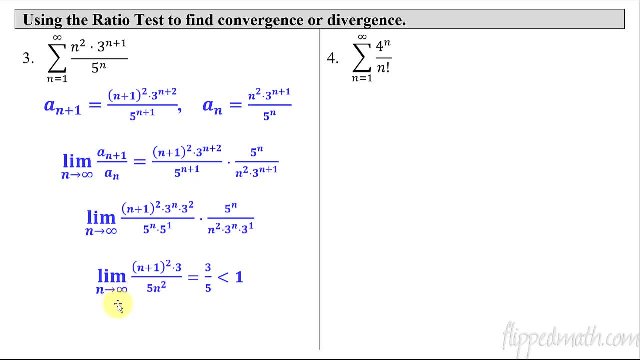 And then I'm bottom 5n squared. So since I'm doing a limit as n approaches infinity, I'm just looking. OK, I've got an n squared and n squared, So I'm just doing leading coefficients And that is 3 fifths. 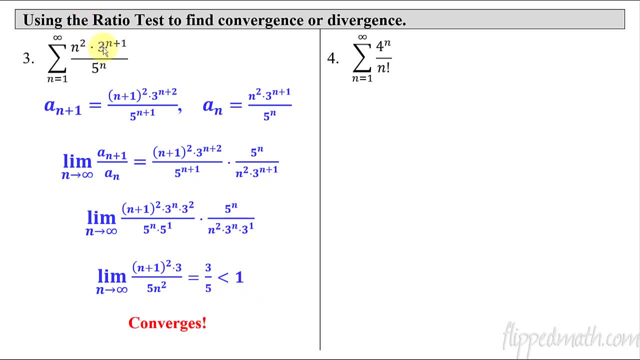 And since 3 fifths is less than 1, that tells us that this series converges. OK, so I know I'm doing this kind of quickly. Hopefully you can follow along, But you can always pause and write stuff down if you need to. 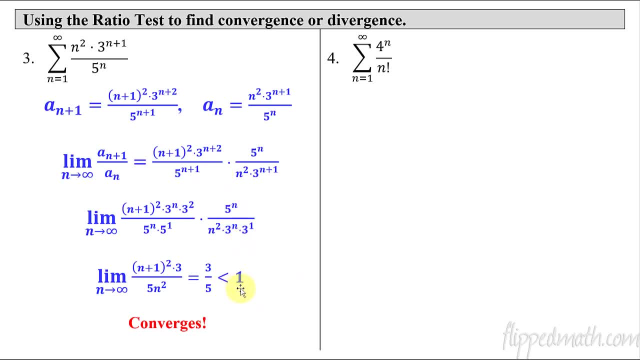 So that was the ratio test for this. Since it was less than 1, it converges. All right, now let's use the same type of thing, But now we're going to have some factorials going on here. So we write out the a of n plus 1.. 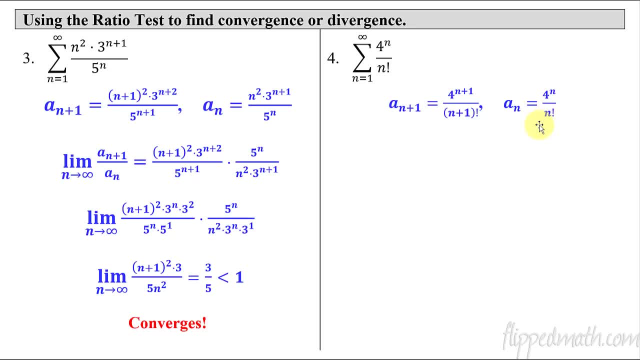 So plug that into the n, Plug that into the n, And then our original. And what do we get from here? We get the limit of the ratio. So I take the a of n plus 1. Multiply by the reciprocal of a of n. 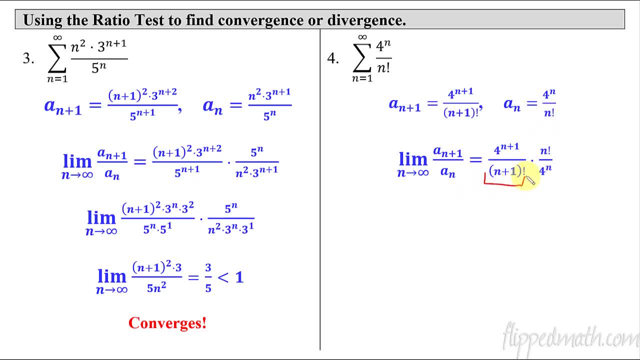 And now that leads us to this where we need to try to simplify that thing. Let's break it up a little bit, So that's where we get this part right here. So n plus 1 times n factorial is exactly the same thing as this. 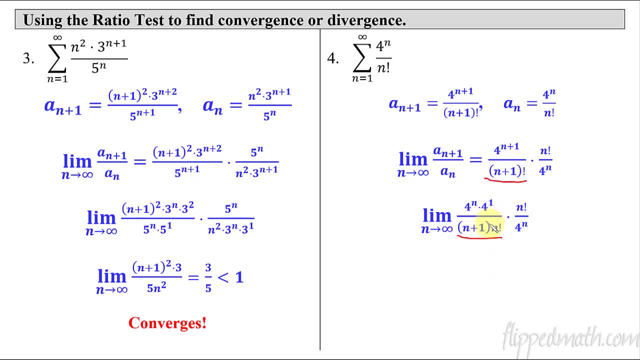 They are equivalent. So once you can see that and break it up And you can see what I did with the numerator there too, How I divided that stuff up, Now I can start canceling stuff. So 4 to the n- cancels. 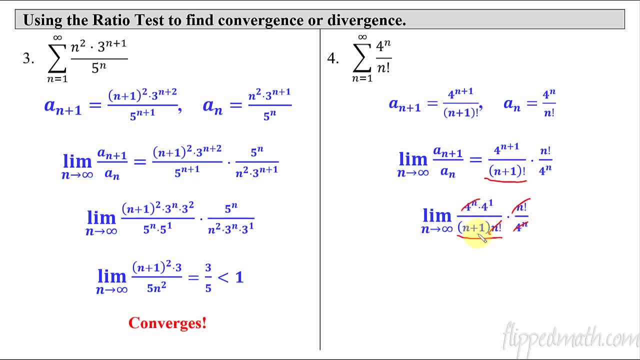 n factorial cancels, And that's really nice. I'm just left with 4 over n plus 1.. So I have the limit of this thing, And that limit is going to equal 0.. Since 0 is less than 1.. 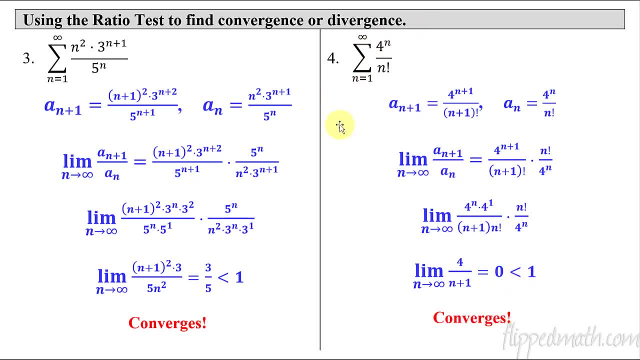 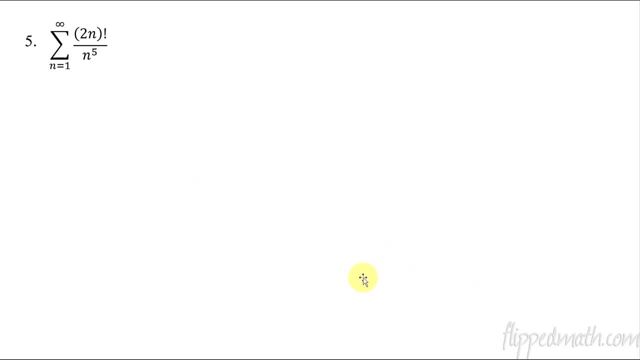 This whole series converges. All right, That is that one with the ratio test. Okay, So let's do one more example, and then we've got it. So now we have one that's a little bit trickier, with 2n factorial on top. 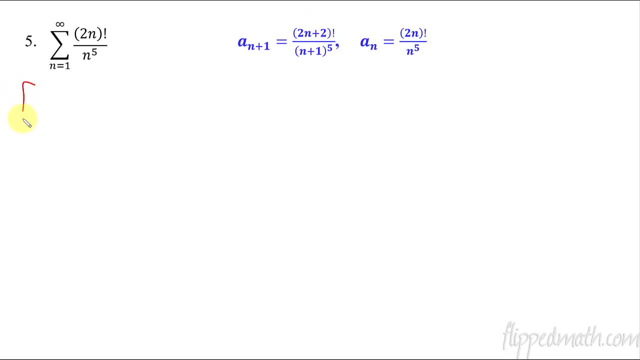 So I've got this 2n plus 2 factorial. If you're not sure where that came from, It's because I have 2 times n plus 1 factorial And then the 2 distributes and gives me 2n plus 2.. 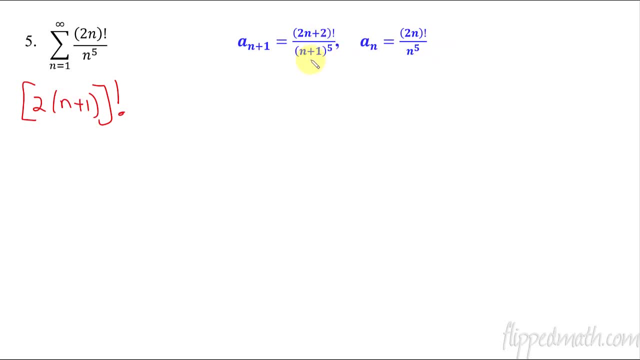 That's where it comes from: 2n plus 2.. All right, So then I've got that. So now let's set up my ratio. I do my a of n plus 1 first times a of n reciprocal, And now I have to get something confusing.